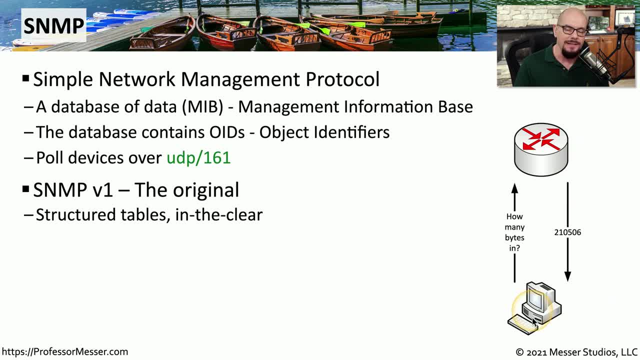 but sent all of this information across the network without any type of encryption or protection. Everything was in the clear and if you were capturing this data with the protocol analyzer, you would be able to see all the queries and all the responses. An updated version of SNMP was created: SNMPv2.. 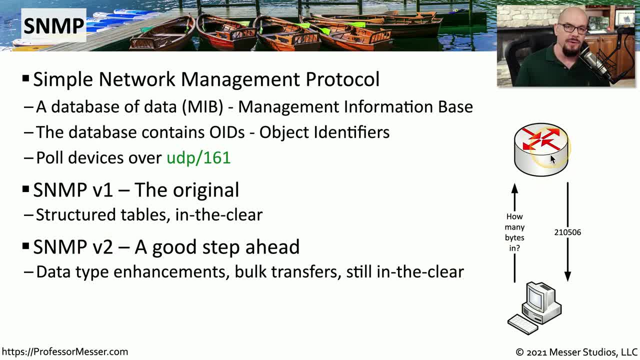 This allowed for some new types of data sources on the remote device and allowed us to query multiple OIDs at the same time and receive all of those responses in one single packet. Unfortunately, SNMPv2 did not include any type of protections either, and everything was sent in the clear, just like SNMPv1.. 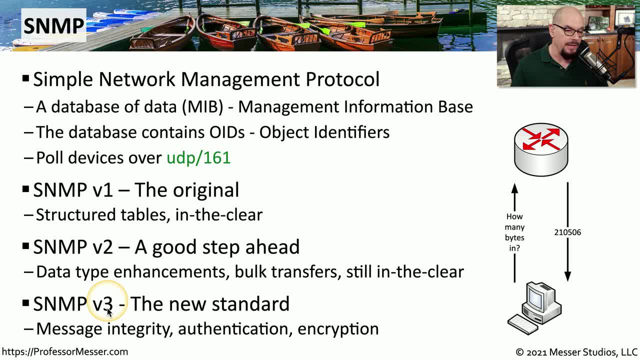 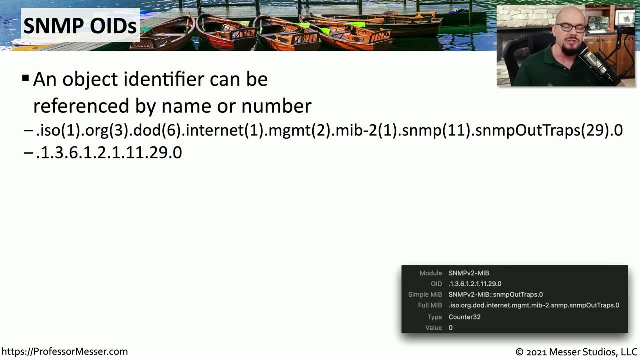 Networks that are concerned about security are probably running SNMPv3.. This includes extensive protections of the data, including a message integrity check, authentication and encryption of the data across the network. To be able to retrieve those metrics from that remote device, we need to know what. 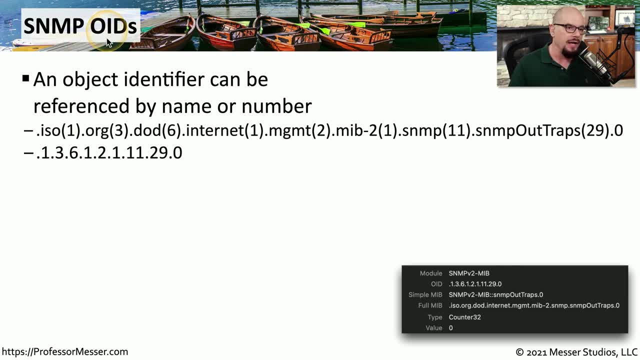 to ask for, and the information that we're asking for is called an object identifier or an OID. These OIDs are a series of numbers. You can see an example of an SNMP OID: 1.3.6.1.2.1.11.29.0.. 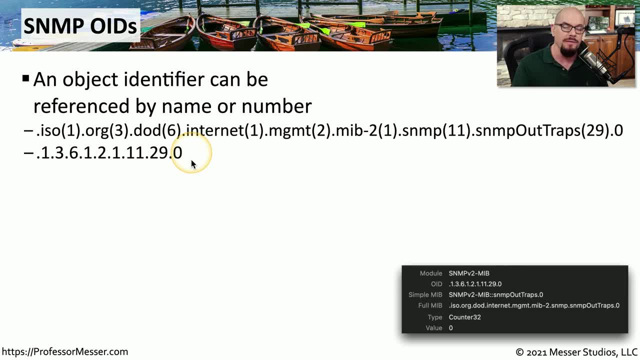 Each one of those numbers is referring to a different part of the SNMP tree. The first number one refers to ISO. the second number three refers to org. third number six refers to DOD. the next number one refers to internet, and so on. 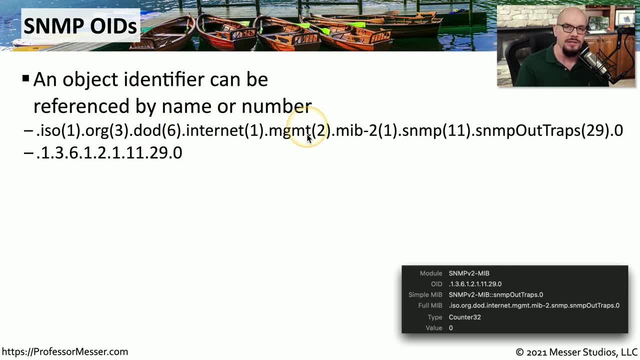 So you could spell out what each of these particular sections mean by their number, but when you're sending this information across the network, all you're sending is a series of numbers. This means that you could have a very large management information base that contains hundreds or even thousands. 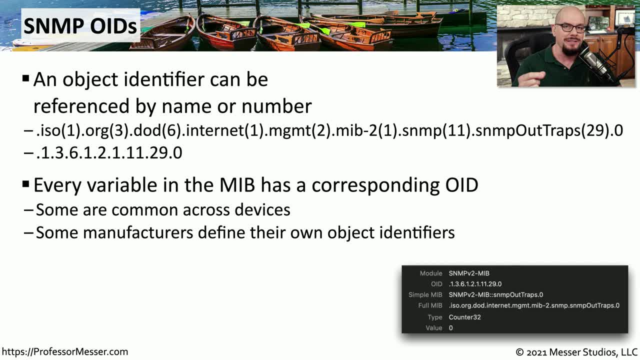 of OIDs that you could reference, You have to be sure that you're requesting exactly the OID that you need to be able to receive the information back from that device. And not only are there well-known OIDs that you could be referencing, but some manufacturers. 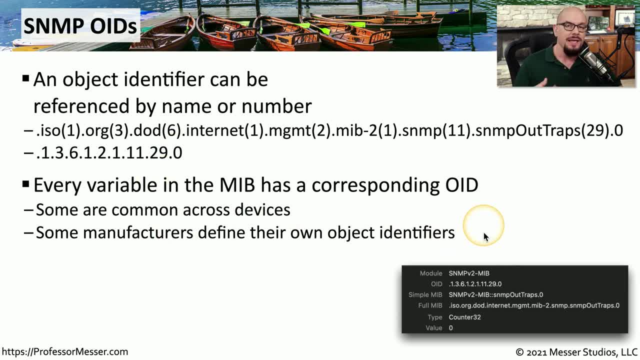 will define their own private management information bases that have their own set of OIDs that you have to know. Usually these proprietary MIBs are documented by the manufacturer and you can usually integrate those into your management workstation. This allows your management workstations. 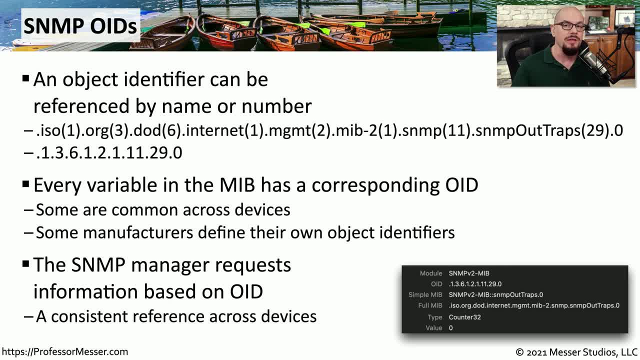 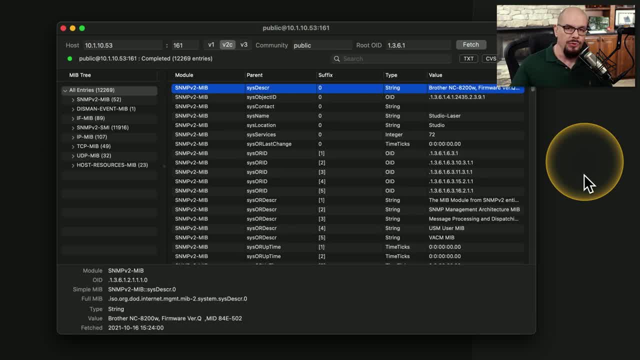 to have a standard query that they can perform, knowing that they're receiving exactly the type of information that they need. What, With the right software, you could even walk through the MIB. This is a MIB walking application that allowed me to query one particular IP. 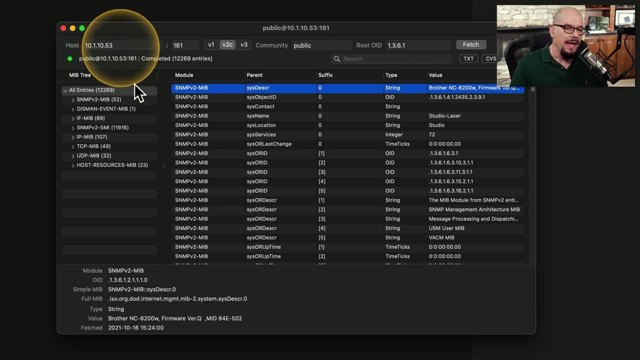 address on my network, 10.1.10.53. And in that device I found thousands and thousands of OIDs all within different management information bases on this device. Now we can see the very first one that was gathered was a system description OID. 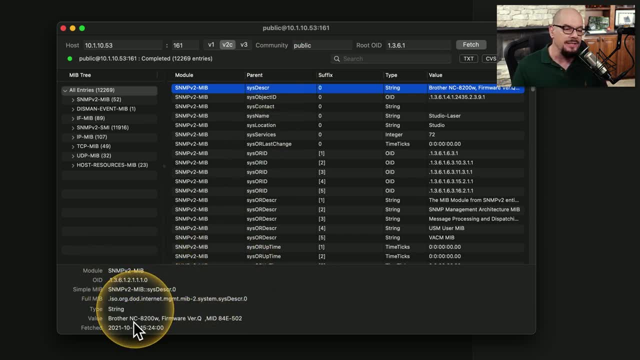 You can see the letters and numbers associated with that And you can see that it is a brother NC8200W firmware version Q, which means that this particular device is a laser printer on my network. As you can see, there is an extensive amount of information. 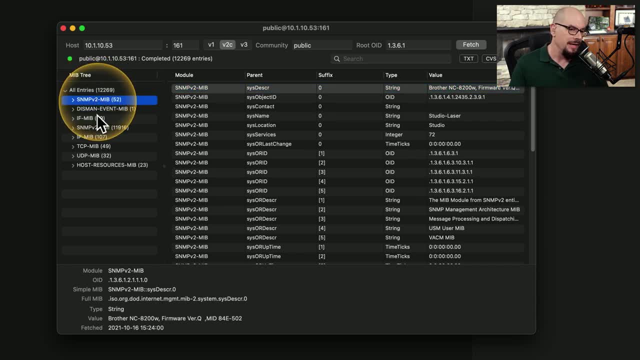 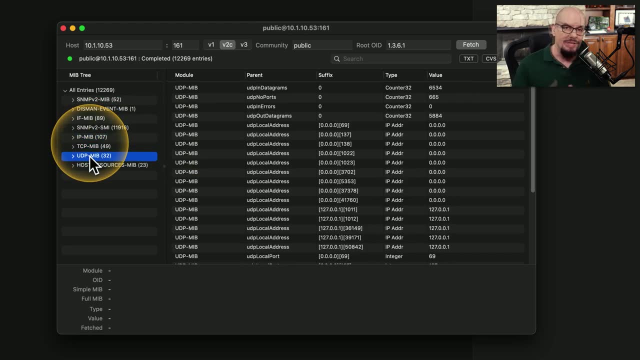 that we can gather from this device. There are SNMPv2 MIBs, there are interface MIBs, there are IP MIBs and some MIBs specific to TCP and UDP. In some cases you may have to walk through the MIB. 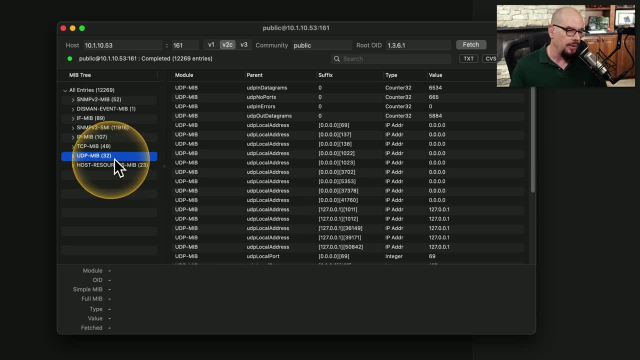 to find exactly the information you're looking for, at which point you could make a note And then you can use that in your management workstation to be able to constantly retrieve that data. If you do that, you can start creating a trend of this information and be 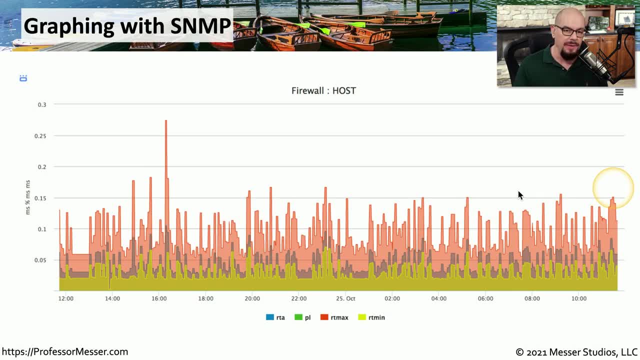 able to compare different metrics over time. This is an example of the information that you could gather over time and create some graphs based on these well-known SNMP MIBs. So far, we've described this SNMP process as very proactive, which means we 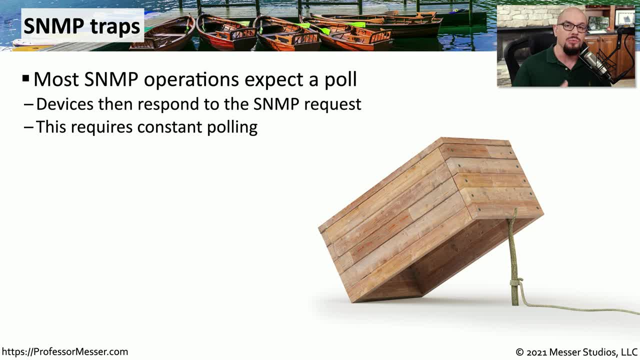 have to query the device and we have to do that in a very specific way. So let's get started. So we have to go back to the device. It responds back with a value, and then we would need to perform trending of that value over time. 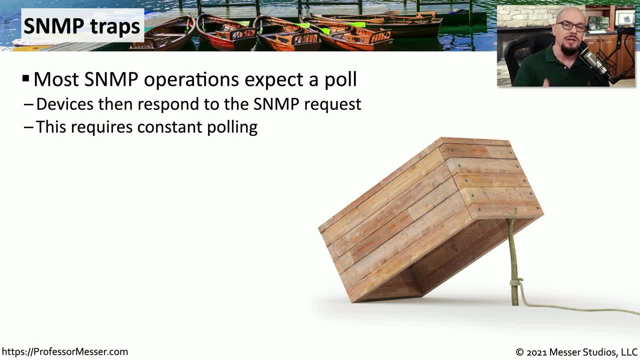 This obviously means that we would need to constantly perform polling to that device to be able to collect and trend that information. And if you have tens, hundreds or thousands of devices, you may find it increasingly difficult to be able to perform all of these polls. 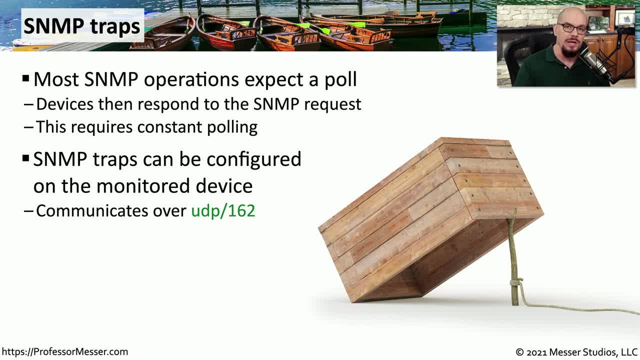 Instead, we could configure the remote device to be able to perform. And if we could configure the remote device to be able to perform these polls, we would have to do a lot of testing and monitoring And, when it exceeds a particular value, to send an alert message directly to us instead of us.